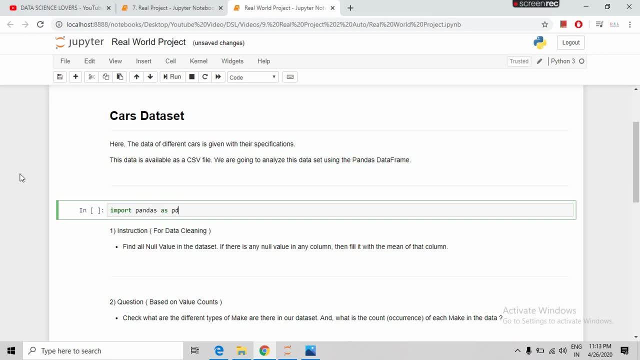 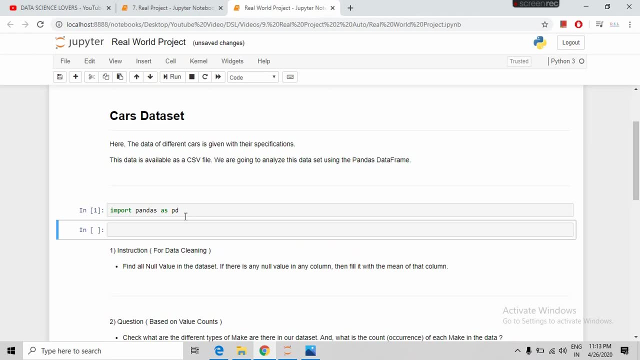 Import pandas as pd. Now, as you can see, the library has been successfully installed. Now we will import our data. Our data is of car, so we will name it car. So the syntax to import a csv file is pd dot read underscore csv, and here we will write the path of our file. 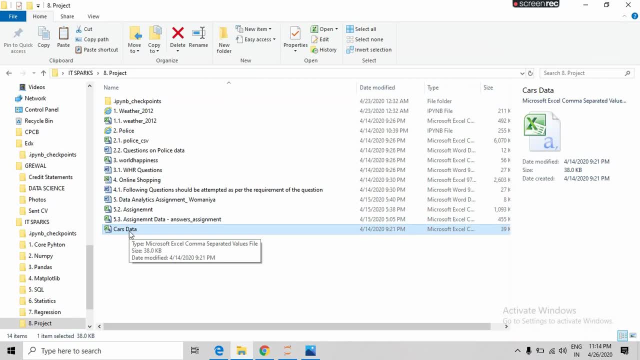 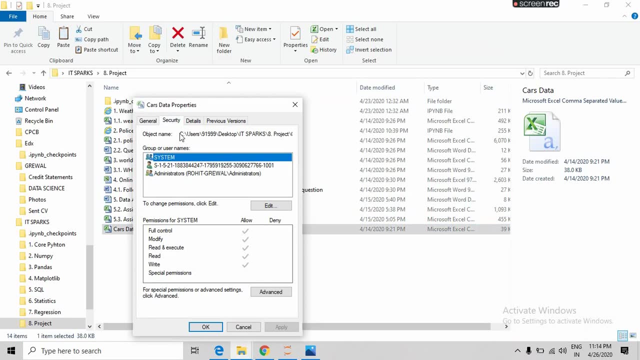 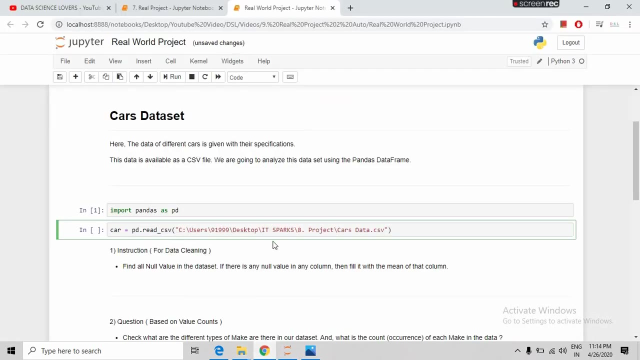 So we will go to our excel. file means csv file, and copy is path. This is the path of this csv file. We will copy it and paste there. Now, friends, I want to tell one thing. If I run this, then it will show a unicode error. Let's see. So it is showing a unicode error. 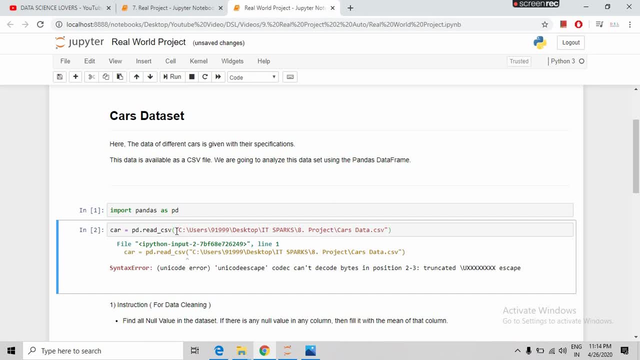 So this happens most of the times. To remove this error, you have to simply write a small r here every time, Whenever you receive this error. So if we run this command, then the error has been evoked and the data has been imported successfully. 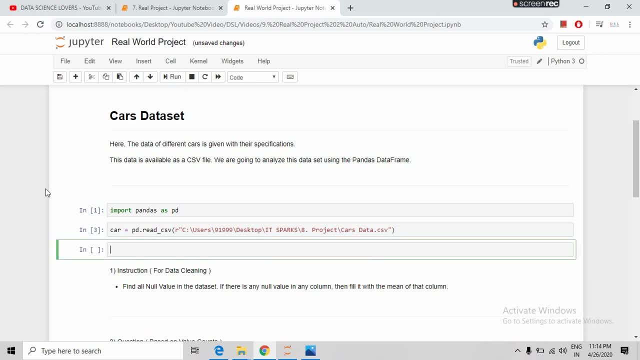 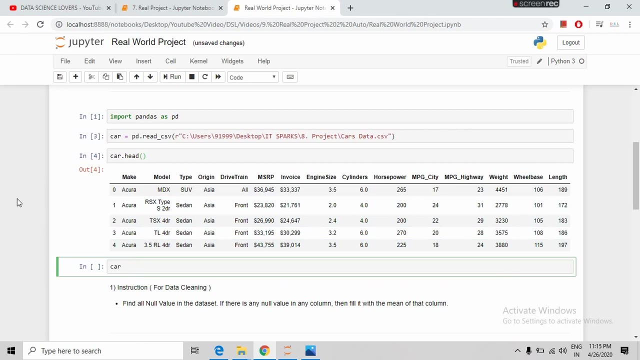 Now to have a look at our data. we will use our data frame name, which is car, here, dot add. If I run this, then this is it. Now we will have a look of the number of rows and number of columns present in our data. 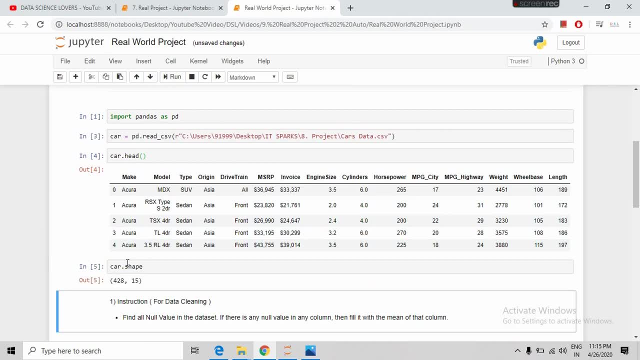 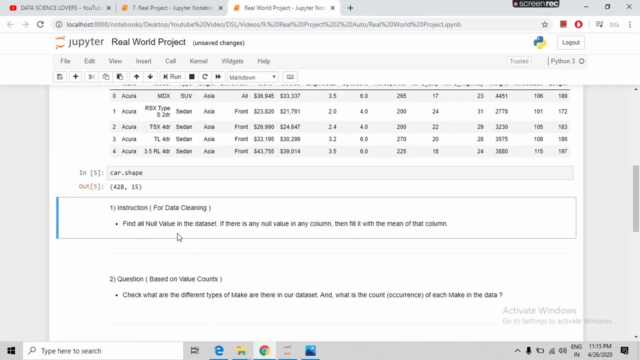 So we will write the command shape. So in this data there are 428 rows and 15 columns, As you all know. these are the rows 0, 1, 2, 3, 4, and these are the columns make, model, type, origin. So, friends, 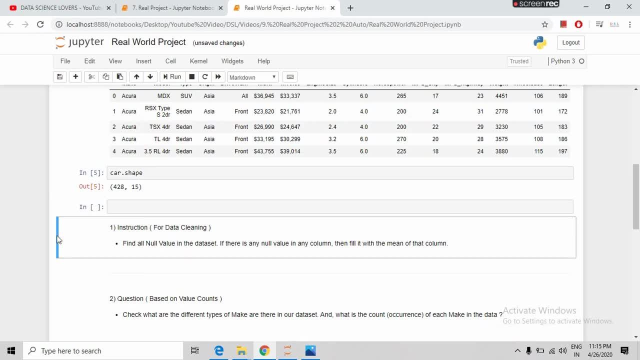 our first question is related with data cleaning. If your manager asks you to clean the data, then he may ask: find all the null values in the data set. and if there is any null value present in any column of the data, then fill it with the mean of that column. So how we will. 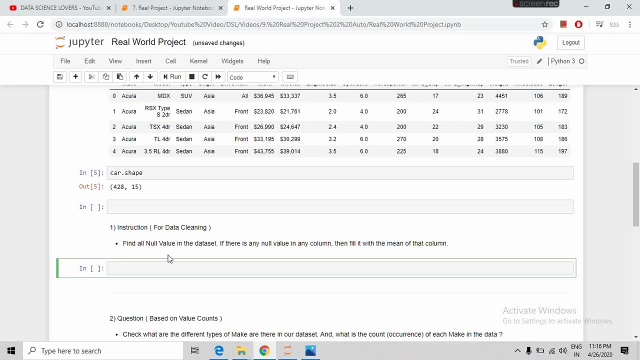 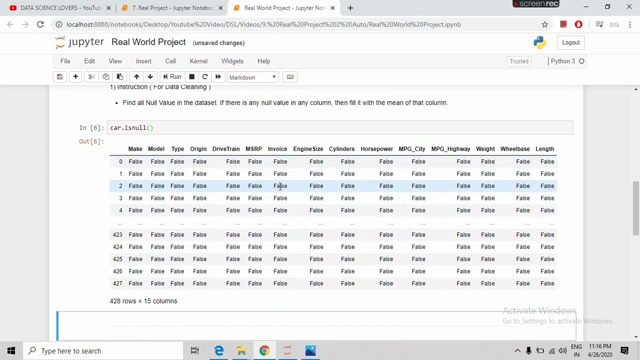 solve it, Solve it. We will first of all see see how many null values are present in any column. the syntax is our data frame name, which is car. here, dot is null and function is null. function is used to check the number of null values present in the columns. if i run this, then it is showing the in the form of volumes. 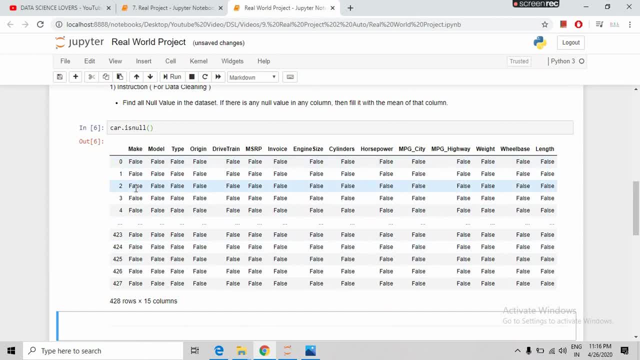 means true or false. false means no null value is present here, and if there is any true, it means null values are present there. so as of now, we are not seeing any. null value means no true. and if i use sum function at the last of the syntax and run it, then it: 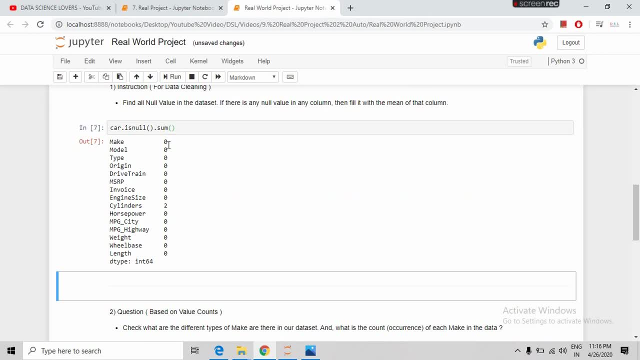 will show in this format means the first column make has no null value. the type column has no null value. no null value. here is a column cylinders which has two null values. so we have done our first part of the questions. find all the null values in the data set means there are two null values only. 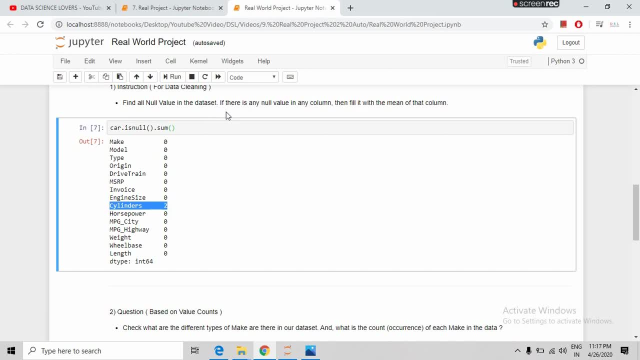 which are present in the cylinder column of our data set. now we are asked to fill the null values with the mean of that column. so these two null values we have to fill with the mean of cylinder column. so to do this we will write a simple command. first of all we have to work on our 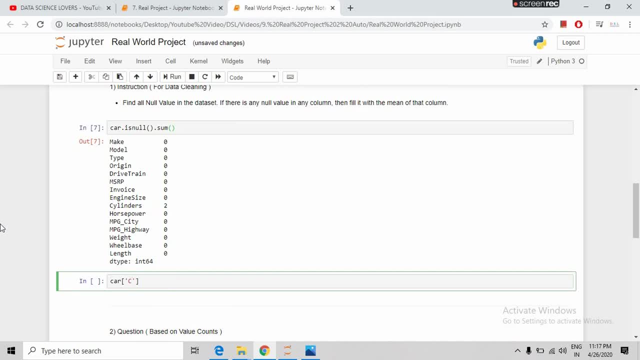 cylinder column. so we will mark our column. this is the syntax for selecting a columns. the syntax is our data frame name and in the brackets we write the column name. so we have to work on this column and the command to fill the null values is dot fill na. and what with what we have to fill? we have to fill the mean. 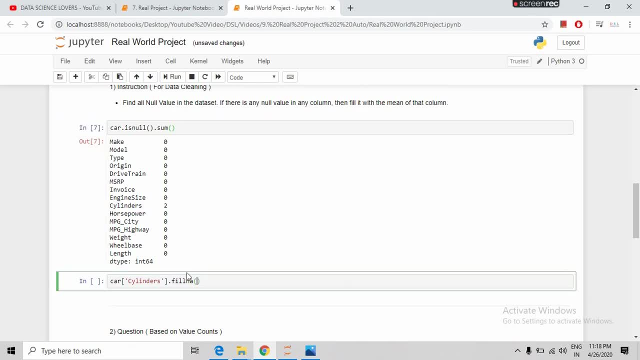 value of the cylinder columns. so again we have to select our cylinder column and its mean value. so to get the mean value we will write mean function. now this is the syntax for this column, so we have to fill it with the mean of that column. so if i run this command, 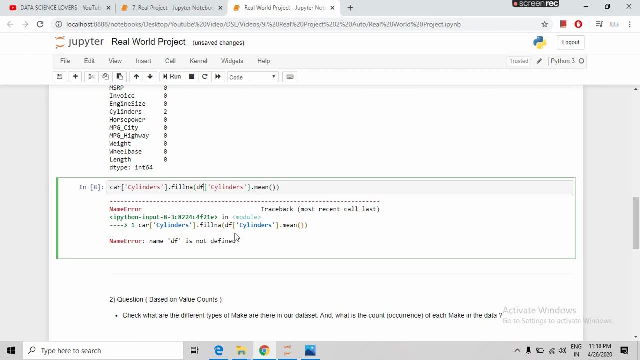 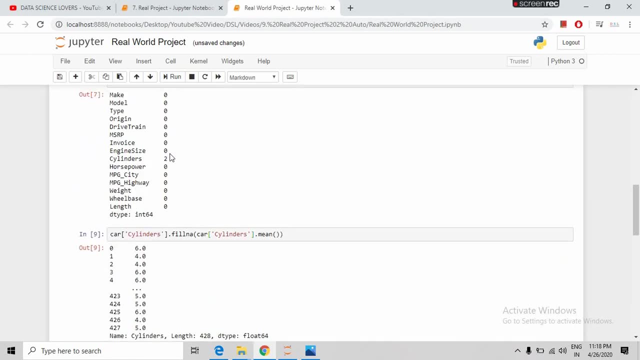 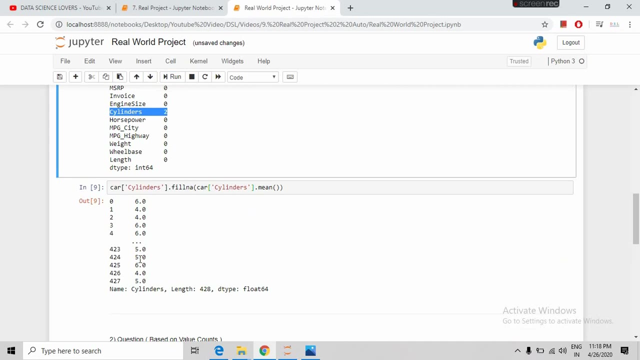 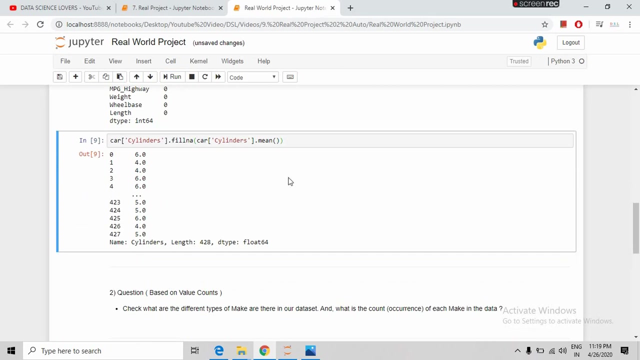 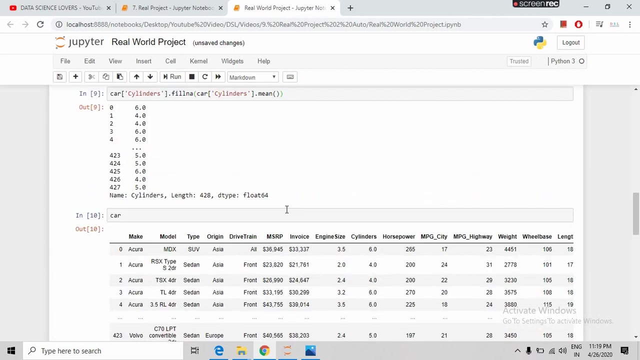 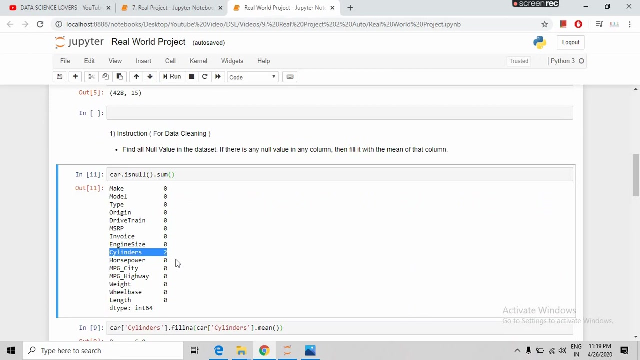 then, sorry, df, i have wrote, i have to write a car, so the two null values which were present in this column has been filled with the mean value. we can't see it here. so now if i run our data frame again and i run this same command, then it is showing that the column still has two null values. 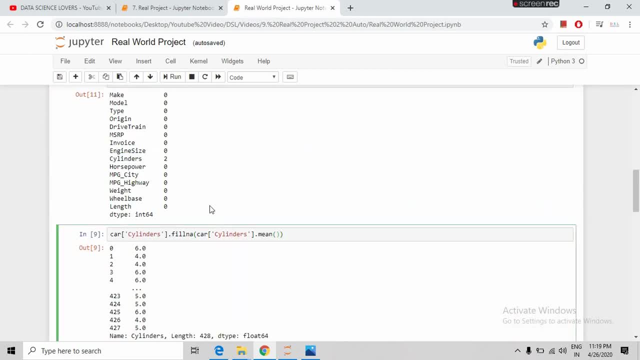 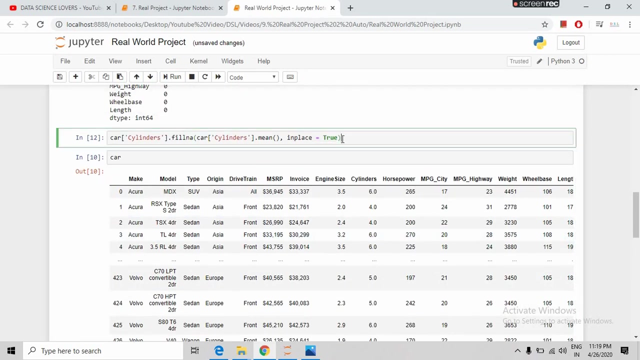 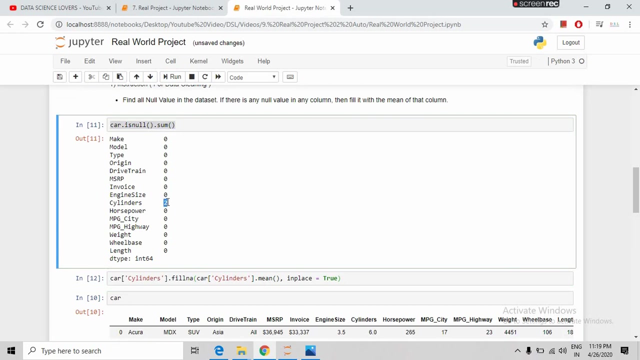 so to make a change permanently. i am telling you one command which we have to write. you have to write in place equal to true. So the inplace equal to true is used to make the changes permanently. So if I run this command, then the command has been executed. And if I run this is null command again, then the 2 will convert it into 0. 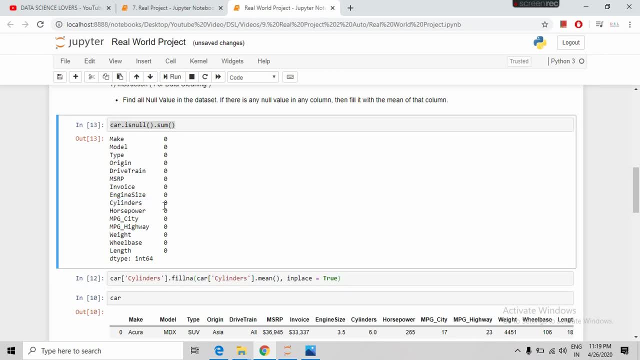 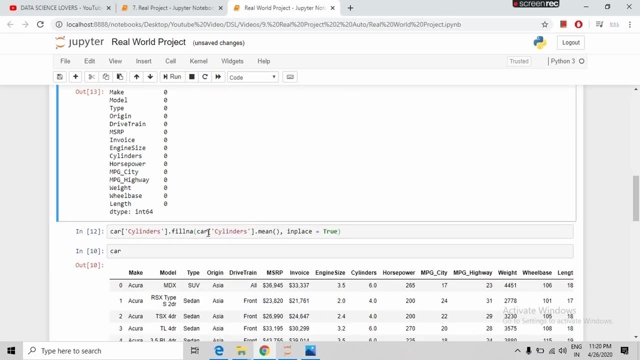 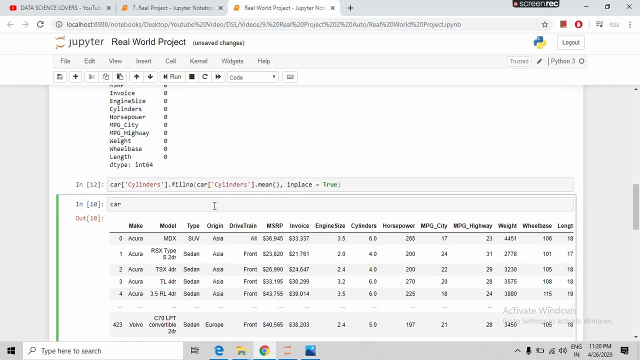 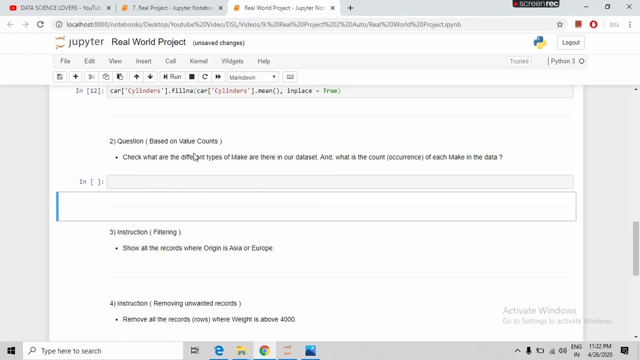 So here you can see that the 2 has been removed and the 2 null values have been replaced with the mean value. So, friends, this was our syntax for this question. So the next question is based on the value count functions. Value count function is a very important function. 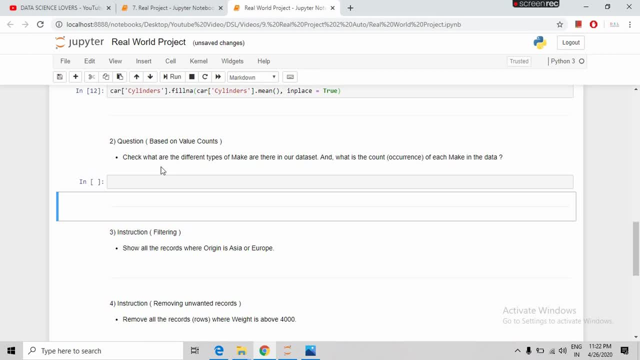 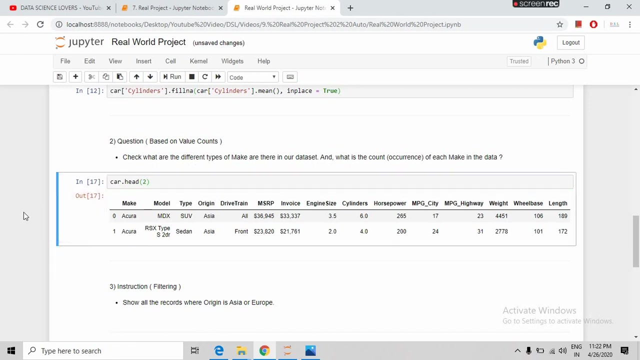 And the question is: check out what are the different types of make are there in our data set And what is the count? Count means occurrence of each make in the data set. So make is our column name. If I show you the first 2 rows, then this is our first column and we have to work in this column. 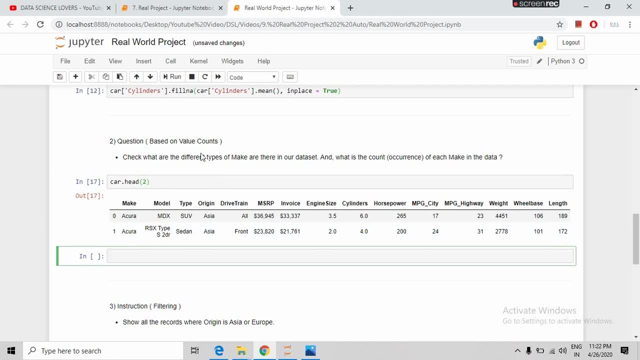 And the hint is given, we have to work with value forms. So we will write the syntax as follows. First of all, we will select our column make, on which we have to work, And we will simply use the value counts command on it. Here we have to write our data frame name, which is car. 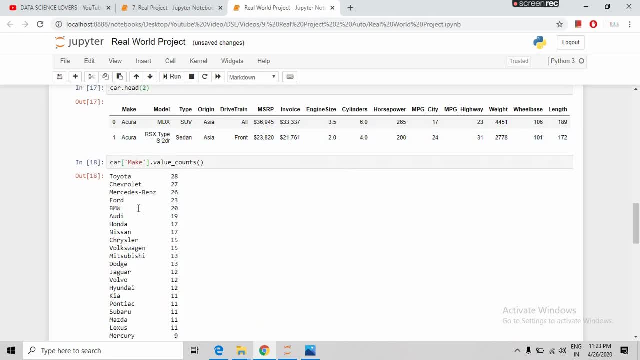 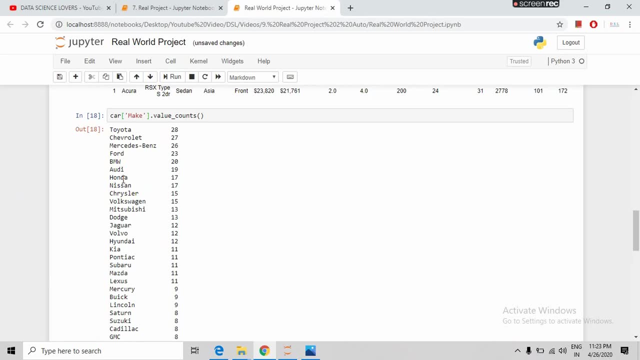 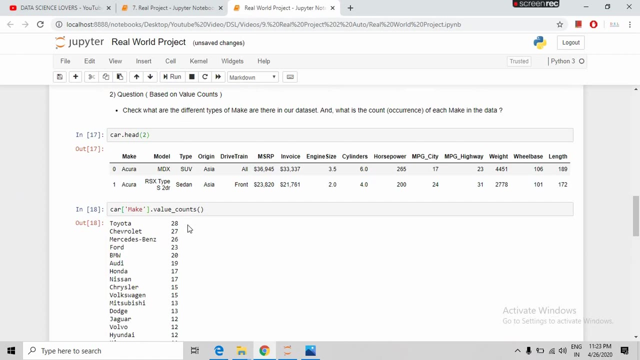 So if I run this command, So here you can see that there are different manufacturers here, Like Honda, Audi, BMW, Toyota, And Toyota has 28 records in total. Ford has 23 records in this data set. Honda has 17 records in this data set. 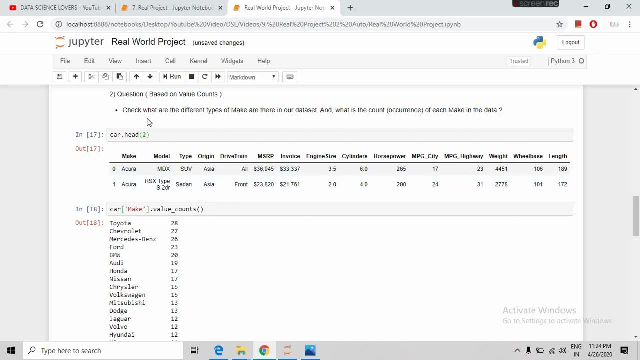 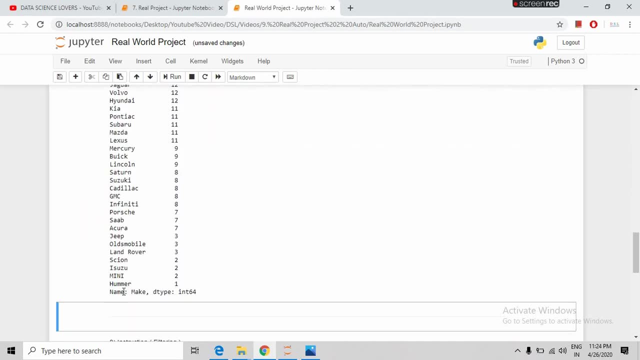 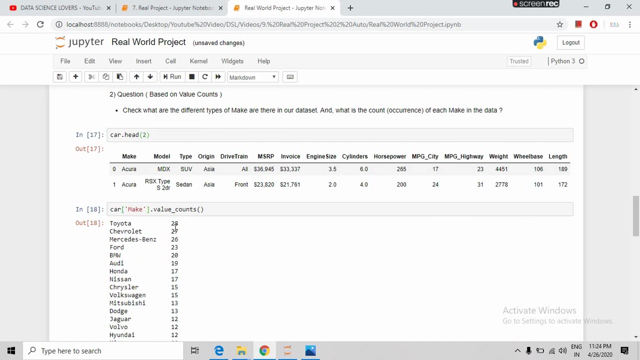 Records means rows. So it was asked that: what are the different types of makes are there in our data set? So these are the different types of makes, Means manufacturer here, And what is the count of each make in the data set? So Toyota is 28.. 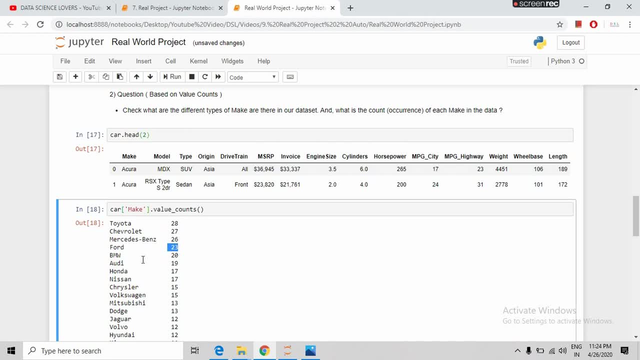 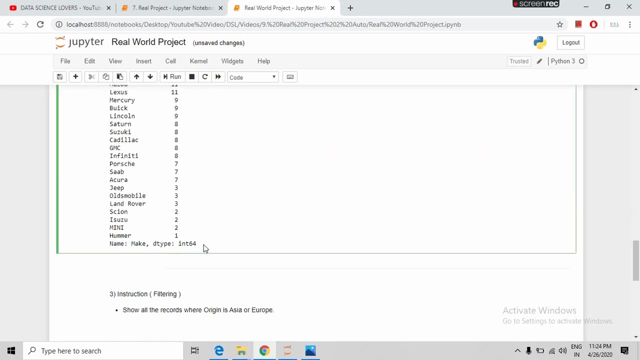 So the count is 28 for Toyota. Ford is 23.. So the count is 23 for Ford. So we have to remember this command Here. it is asking for make column. It can be asked for any column. So if we move to our next question, 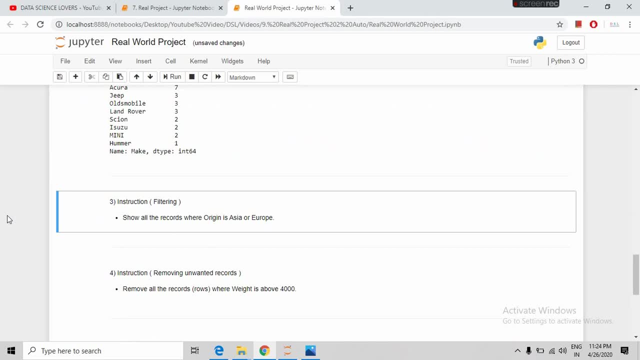 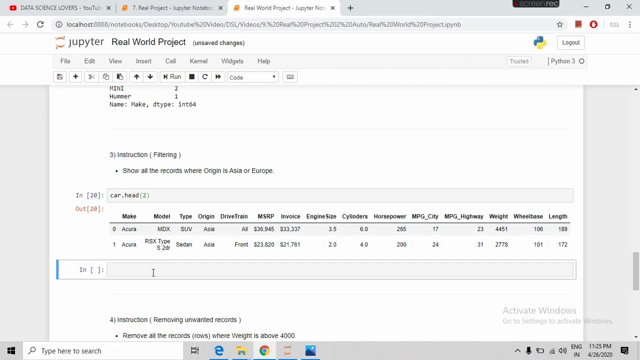 It is based on filtering method And it is a instruction Means someone ask you to show all the records where origin is Asia or Europe. So first of all, we will have a brief look on our data. So this is our first two rows of the data. 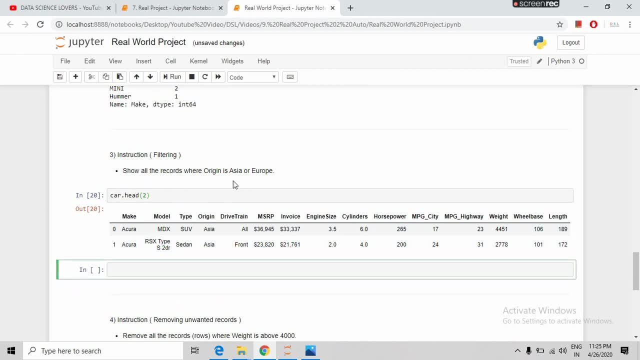 And we have to show all the records where origin is Asia or Europe. In this case, We will use the is in function. Let's see how to use this. First of all, As we have to work on origin column, We will write a syntax to select origin column. 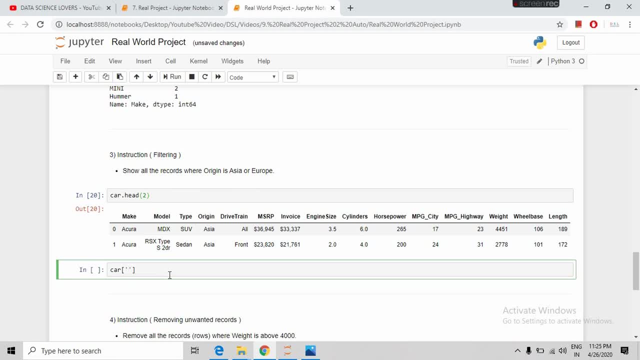 And the syntax is our data frame name And, in bracket, our column name. Now the column has been selected means In this syntax. Now what we have to do, We have to find all the records Which contain Asia or Europe. This is the origin column. 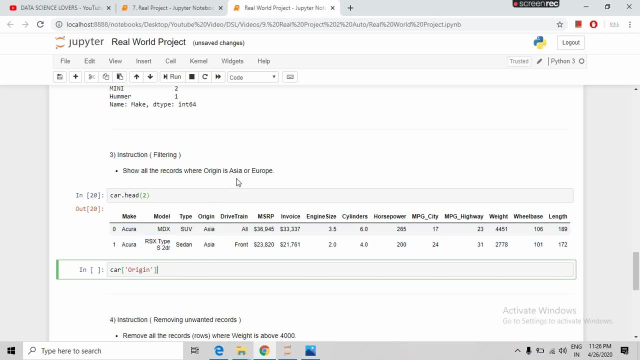 And it has the many records And we have to find only those records which have Asia or Europe. So the syntax is: is in And in the list We have to pass the values or elements Which has been asked in the questions. So this is the syntax. 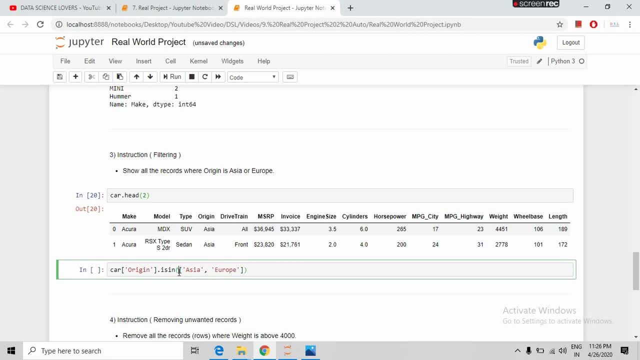 For is in function. Note that all the values that we have to find out Must be written in the form of list. This bracket And this end bracket shows the list. Now, as we have to show all the records, We will write our data frame name here again. 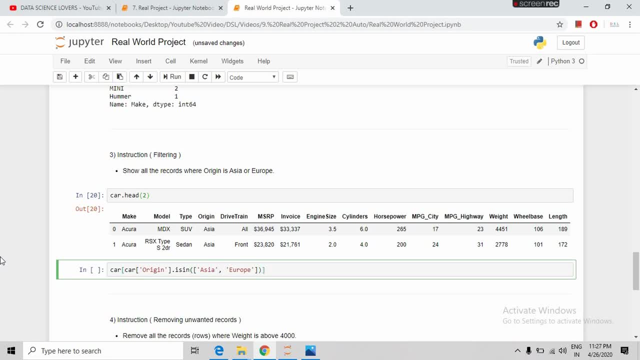 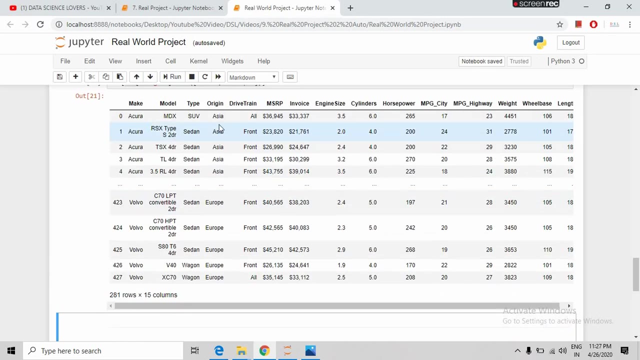 And in the square brackets We will write this syntax. This syntax, All syntax, has to be written In the square bracket To show the records. If I run this, Then it is showing all the records Which have origin Asia or Europe. 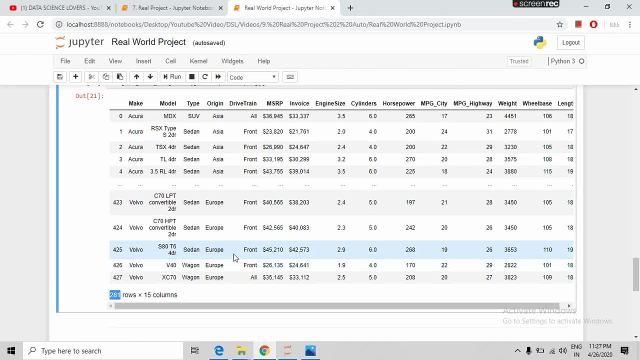 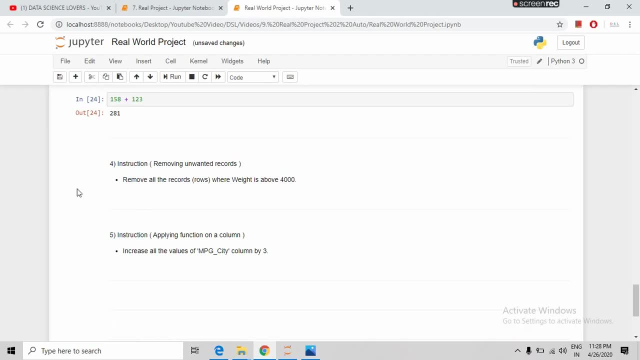 There are total 28 one row records. If we move to our next question, It is asking for removing the unwanted records. If your manager ask you to remove all the records That contain a particular value, Then what we have to do In this question it has been asked. 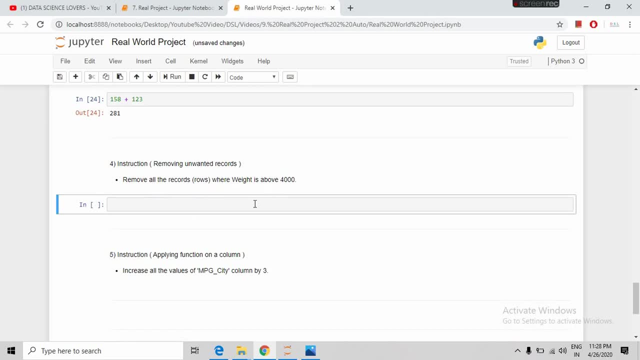 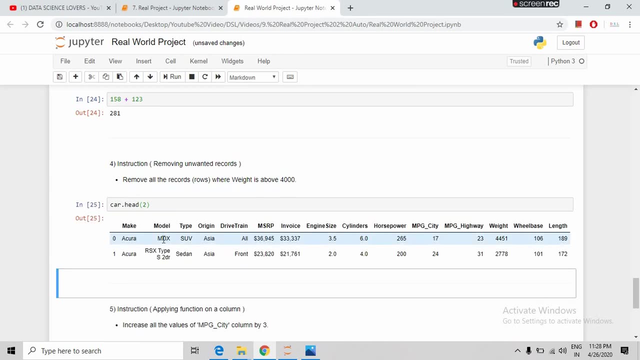 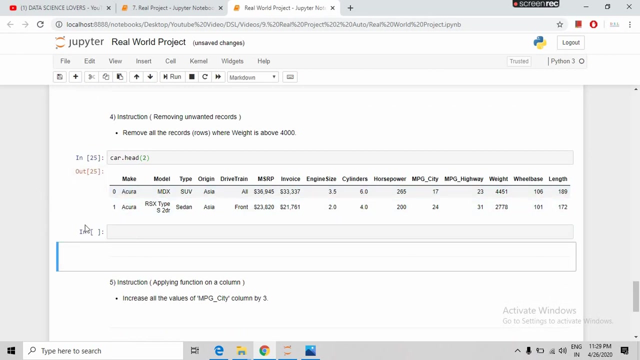 To remove all the records or rows Where weight is above 4000.. First of all, we will have a Look at our data again. This is our data. I am selecting only two rows Here So as I have to work on the weight column. 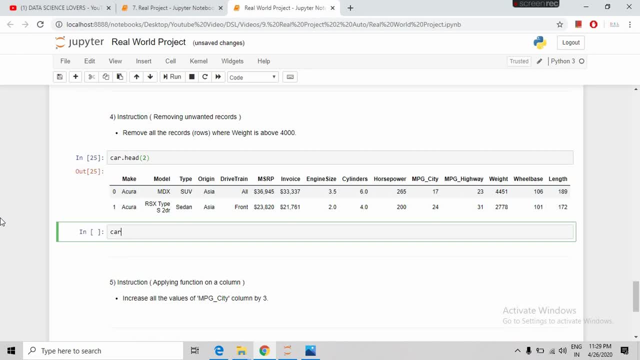 I will first select the Column. So I am working on weight column. So I am working this: Now we have to find all the entries Which has weight greater than 4000.. So If I run this syntax now, Then it will show the result in the form of true or false. 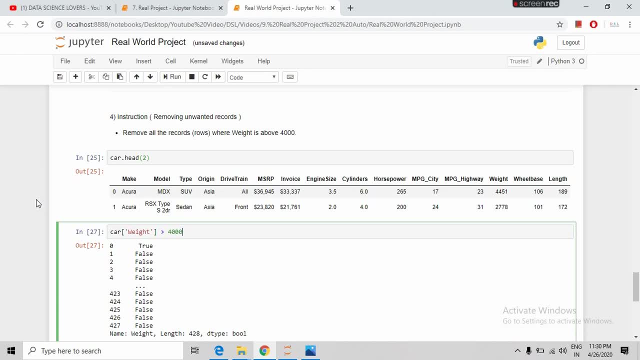 So to show all the records Which are greater than 4000.. We will write The syntax in this format, As I told you earlier That we have to write the Our data frame name And the Syntax in the Square brackets. 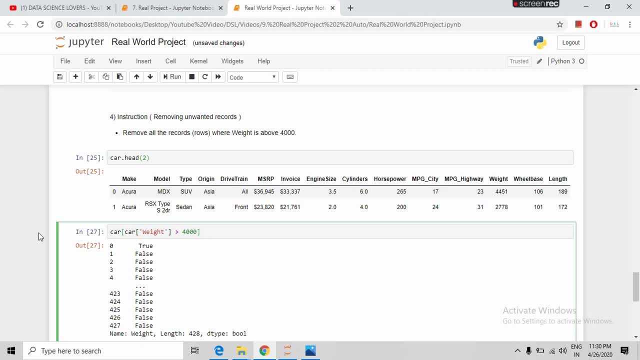 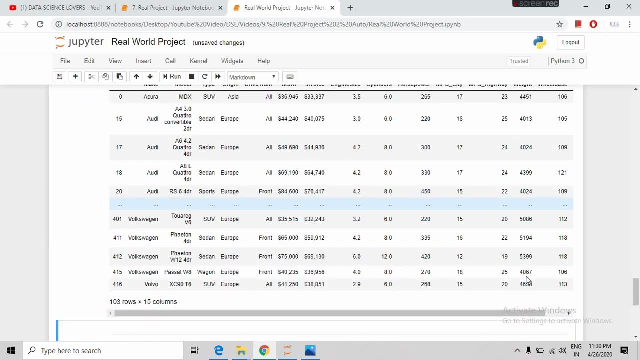 This is the starting of square bracket And this is the end point of square bracket. So if I run this command now, It will show all the records Where weight is greater than 4000.. And the total number is 103.. Now, as we have to remove, 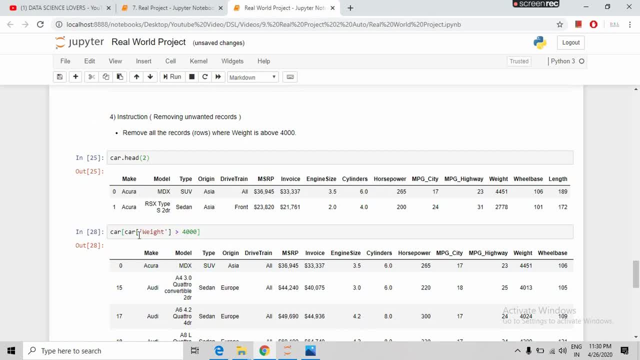 All these records. So what is The syntax that we will use? We will simply Write This sign- Remember this sign- To remove all the records Which contains The weight Greater than 40. Or which contains a specific condition. 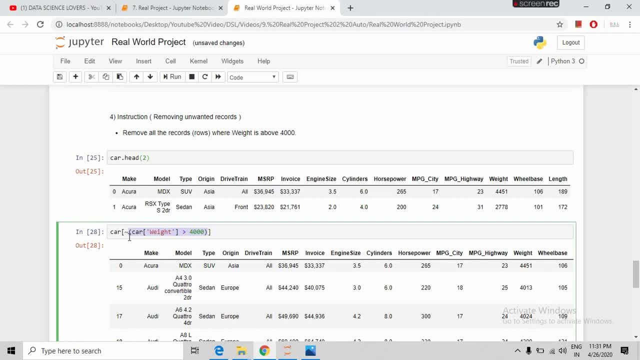 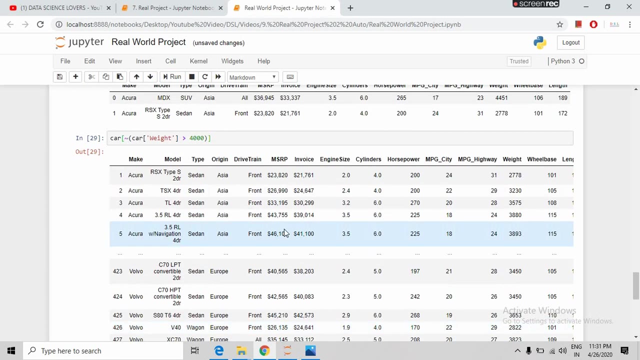 This is the conditions And we have to remove the records Which Shows the Or which specify the This condition. Then if I run this command, Then all the records Have been removed. As you can see, There is no records. 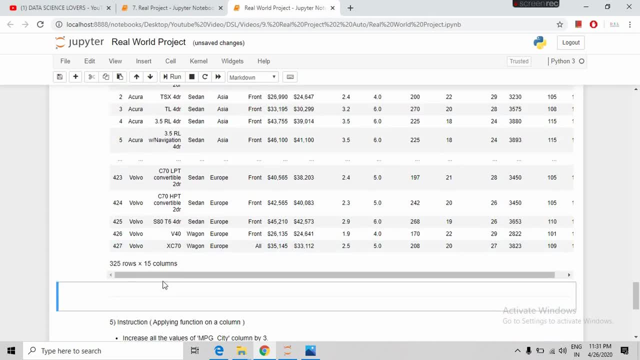 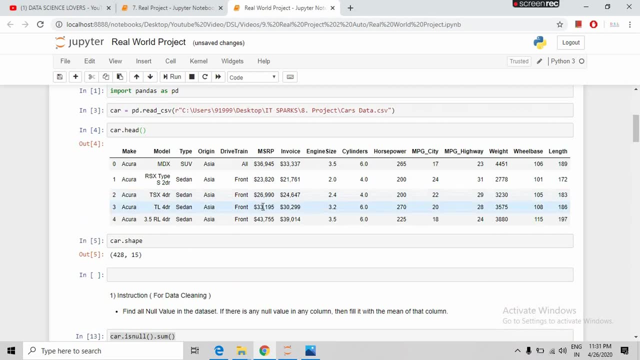 With the value of weight Greater than 4000.. Now, if I have to confirm this, If I See the What was the Data then Shape over data was 428 rows and 15 columns. Now, in the starting we had: 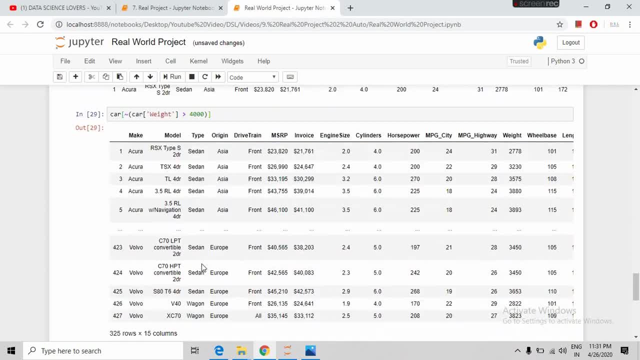 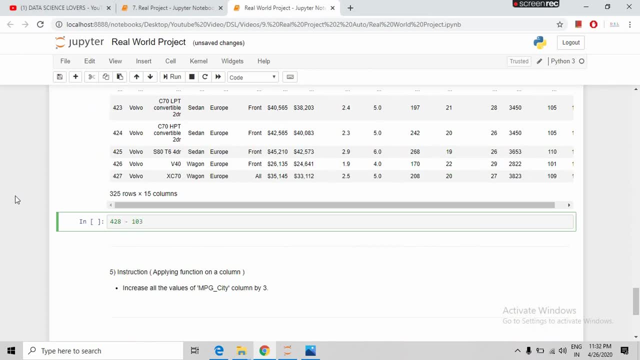 428 rows And, If you remember, There was 103.. Rows Which containing the weight above than 4000.. Now, If I subtract this, Then I will got a value of 325.. And this is the 325.. 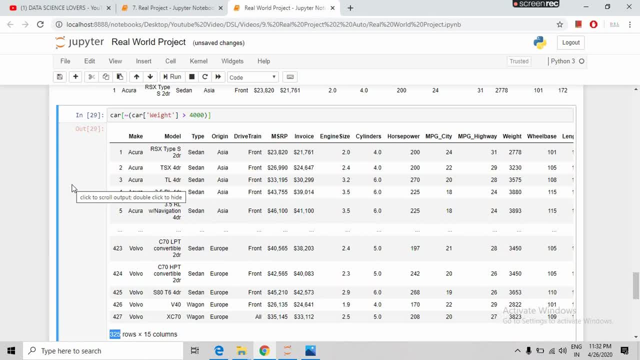 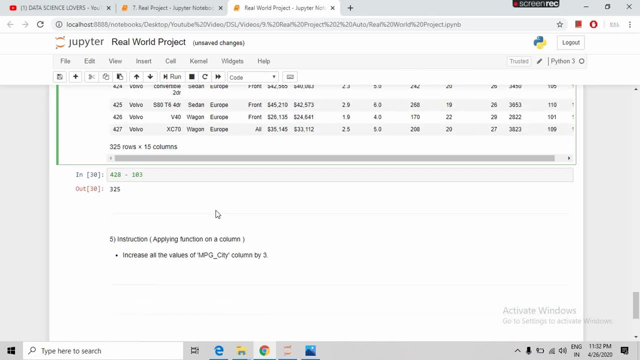 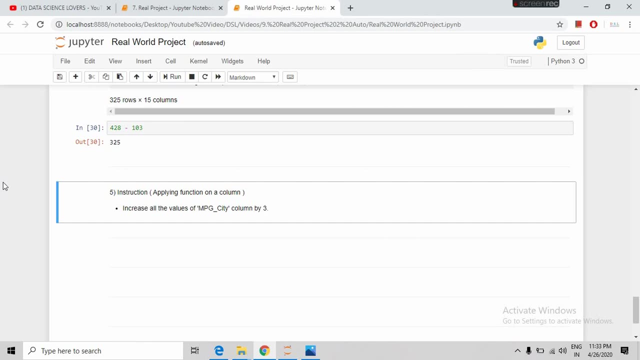 So From the data set, All the records which contain The weight greater than 4000. Have been removed. Alright, Now our next question Is: It is asking for apply A function on a column Now, If we have to make a change. 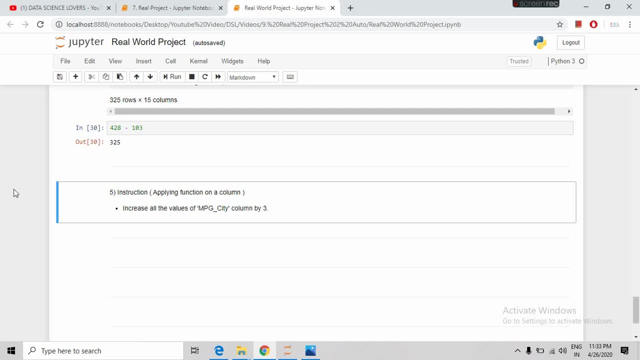 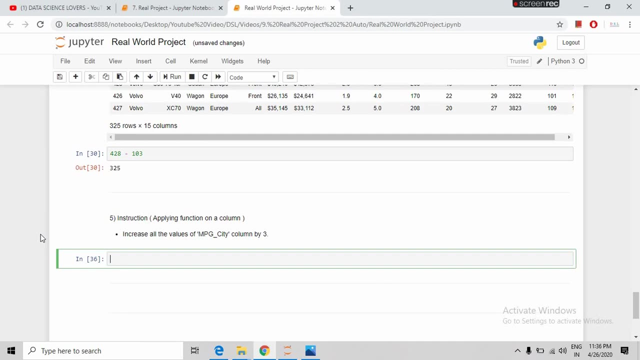 In the values of a column, Then we can use the apply function. Now, How to solve this? We will Use the apply function On it Like this: First of all, we will Have a look at our data frame. This is our data frame. 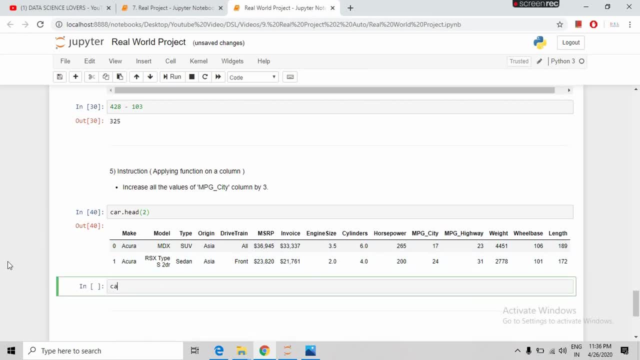 And now we have to work on mpg city column. Then for this We will Select our mpg city column From the data set And we will Use the apply function here In the apply function. You all know about lambda function. 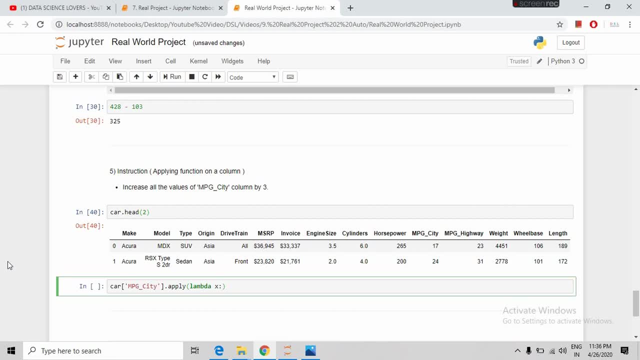 How to use it. So I am using it here. We have to increase the value by 3.. So all these changes We have to made in Car and pg city column. So we will Write our column name here also. 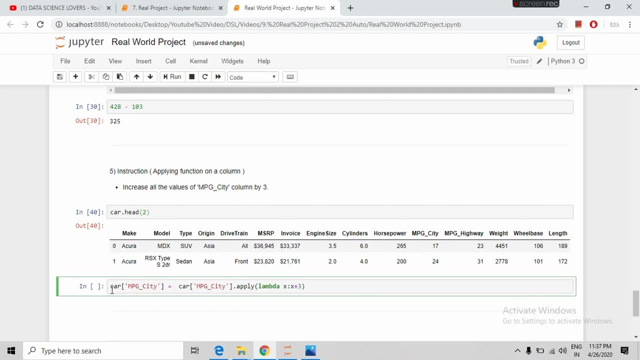 So this is the syntax For this problem Or instruction Or question. you can say In mpg city column, And This is the changes We have to make. If I run this, The command has been successfully Executed And if we have a look at 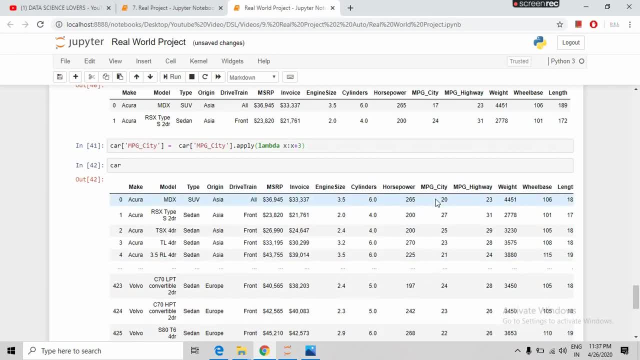 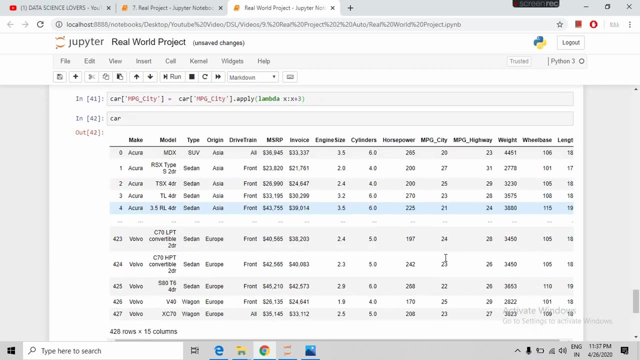 Our data frame. Then we can see that The values has been increased By 3 of mpg city column. Earlier it was 17.. Now it has 20.. The second row had a value Of 24.. Now it has a value of 27.. 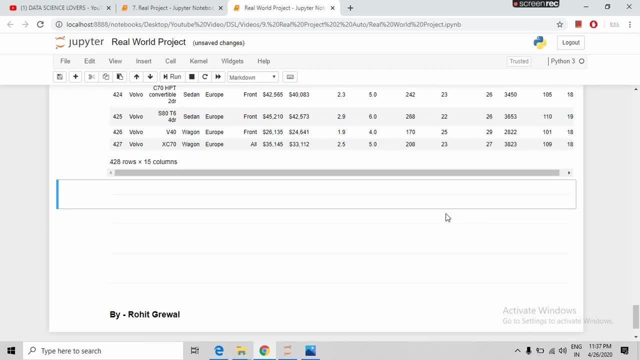 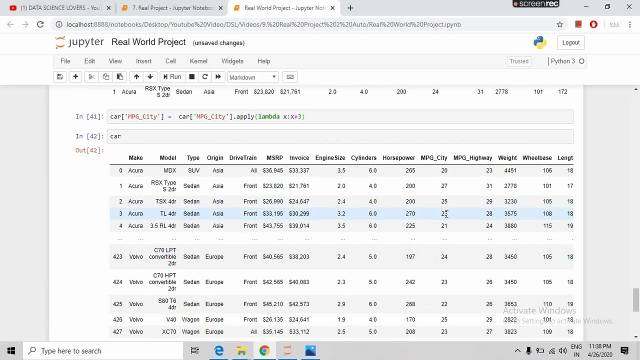 Means, there is a increase of 3. In Each value of the column. So that's all, friends. In our next video We will work on some Other questions On real big data. Thank you, Please subscribe to our channel. 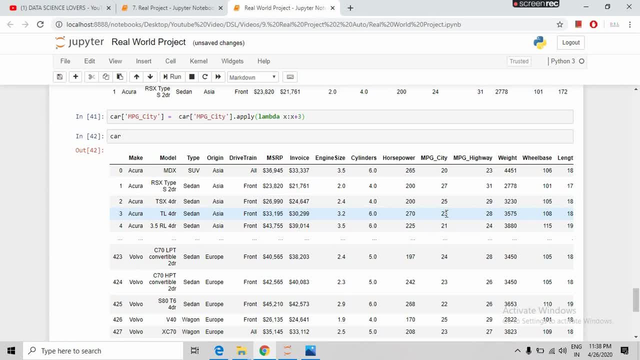 To watch the latest Videos and updates Dated with the Real project working.